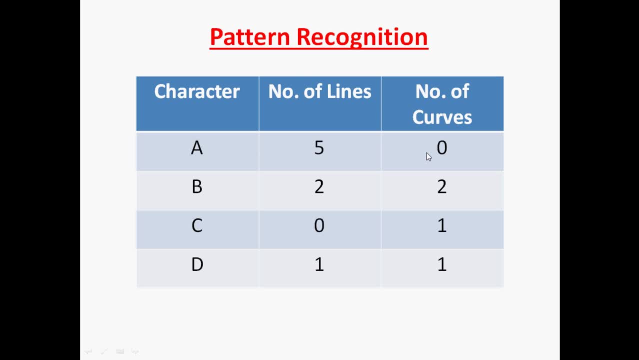 For A, we have five number of lines, zero number of curves. For B, we have two number of lines, two number of curves. For C, we have zero number of lines and one number of curve. And in D, we have one number of line and one number of curve. And this 5, 0 is a pattern of A. 2, 2 is 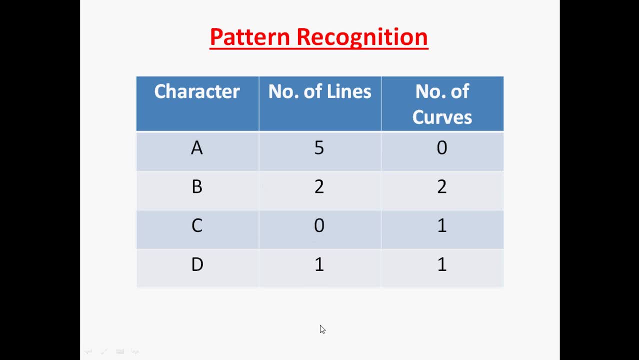 a pattern of B, 0, 1 is a pattern of C and 1, 1 is a pattern of D. Now we can represent this two-dimensional space. We are calling this space as two-dimensional because we have selected two features, So these two features can be represented in a two-dimensional space. 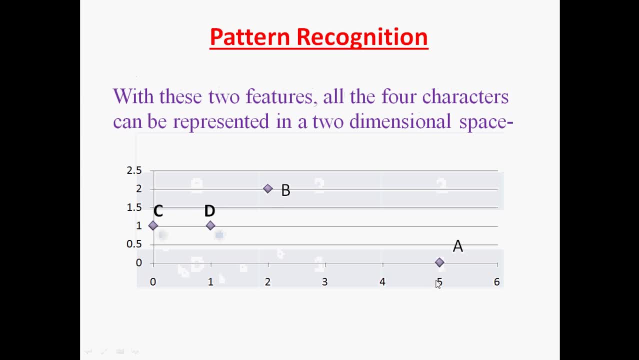 And here we are representing it in two-dimensional space. This A- A is having five number of lines and zero number of curves. So this dimension is representing number of lines and this dimension is number of curves. Similarly, we can say that A is having five number of lines and zero number of curves. 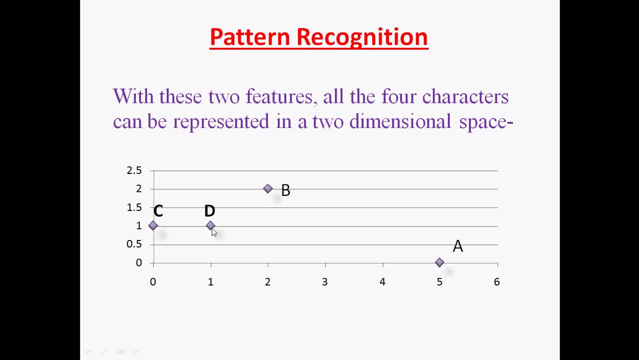 Similarly, B is having two number of lines, two number of curves, D is having one number of lines, one number of curves, And C, one number of curves and no number of lines. No line is there in C. Now suppose someone has drawn this character A and this is unknown. 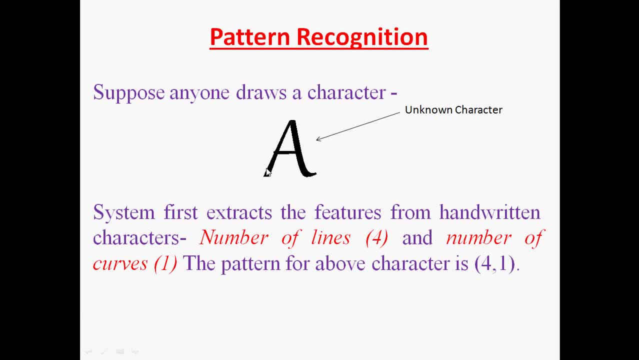 character. We just want to identify this character. Now we say that one, two, three, four number of lines are there in this character And this segment is curved. So one curve in this character and four number of lines are there. So number of lines are four and number of curves are one. Now if we draw, 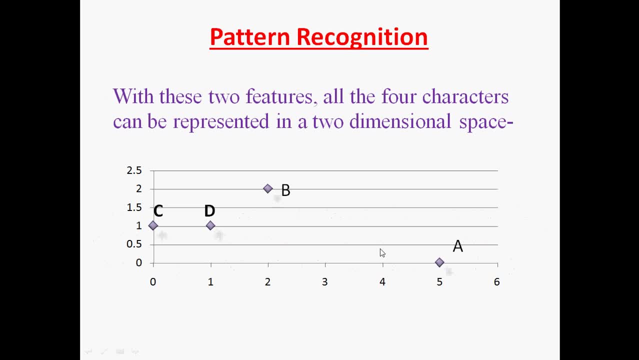 this character in the same space. we see that this character will appear here at this place. Now, this unknown character is nearest to this character. If we calculate Euclidean distance, then this A is nearest to this unknown character is somewhat far. this is away, this is away and this A is nearest character. So we classify. 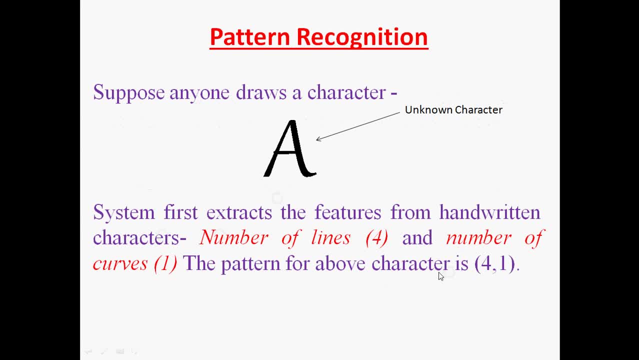 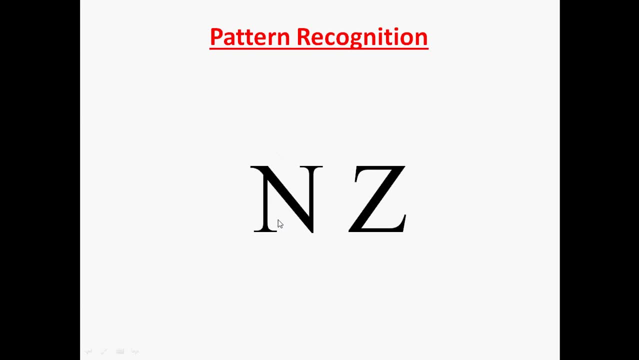 this unknown object as A. But this technique fails when we are talking about N and Z and this does not hold good for all the characters, As we can see in N and Z, in both characters we have three number of lines and zero number of characters, So here it will not work Here.